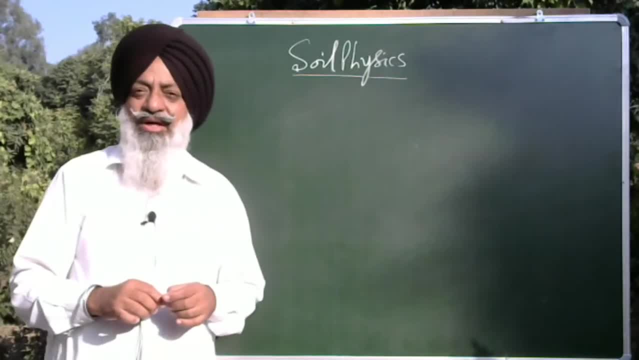 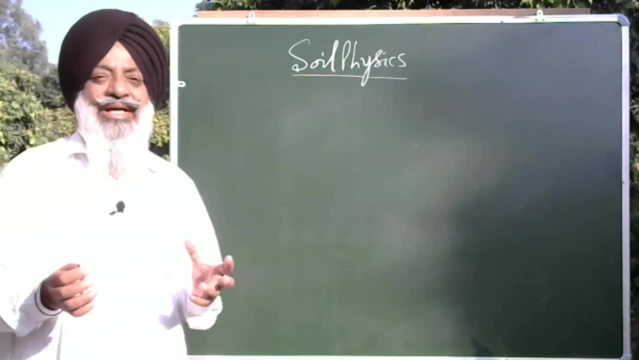 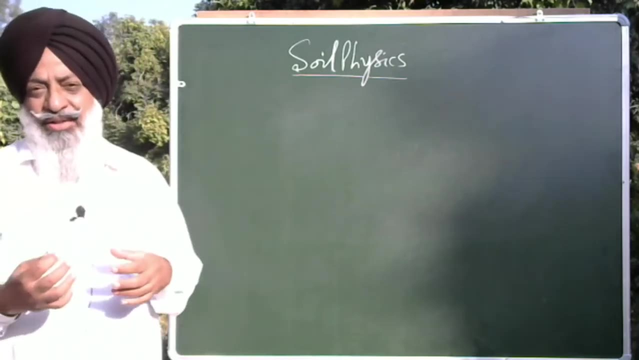 Hello, welcome to my class. Today we will start with an introductory topic on soil physics. What is soil physics? Soil physics, in fact, is that branch of soil science which explains, which deals with soil physical environment. In fact, soil physical environment is very 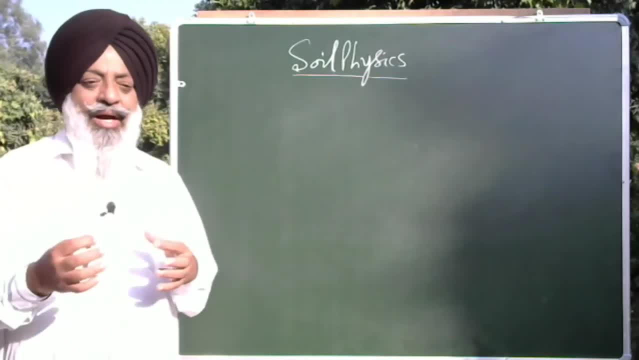 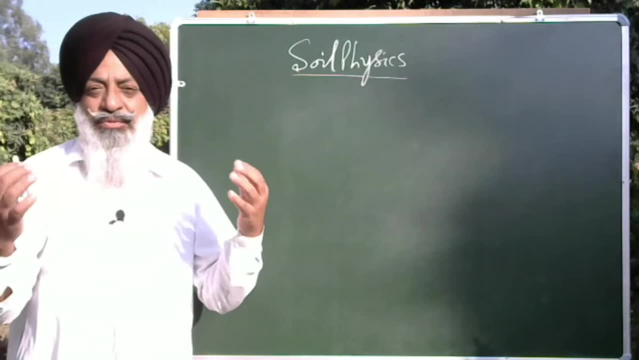 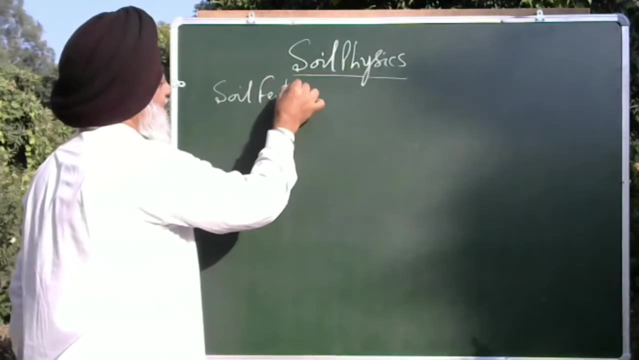 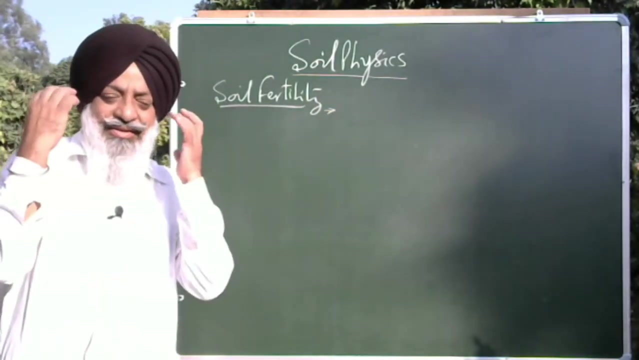 very important for the growth of the plants. Now, in the absence of soil physical environment, let me explain that. what could be the situation? All of you know that soil fertility is the ability of soil to provide nutrients to the plants, And this is the general mindset of the soil scientist, lay persons, even farmers, that soil 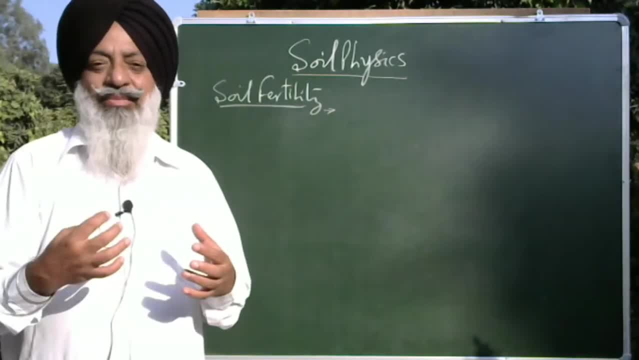 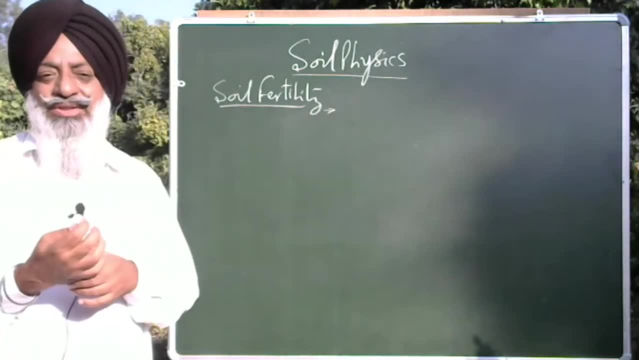 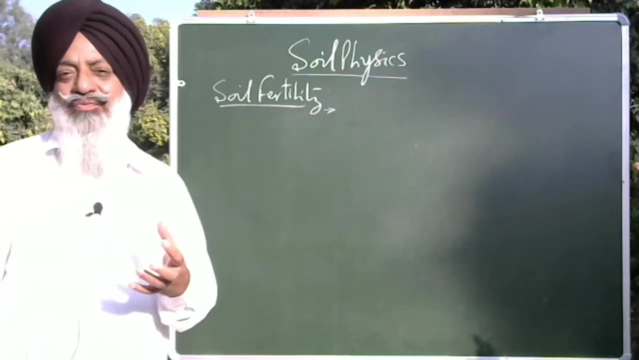 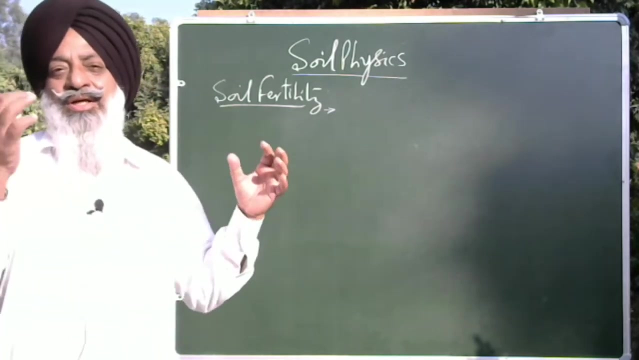 fertility means availability of the nutrients, But in fact the soil fertility is a broader term which is not only includes the availability of the nutrients, But the environment- could be physical environment, could be biological environment, which is important for transforming those elements, transforming those nutrients from soil in one form to another form. 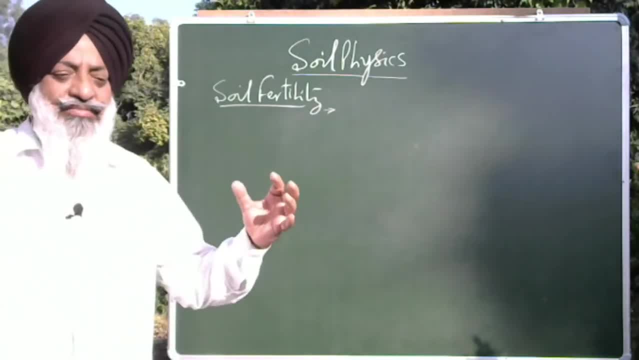 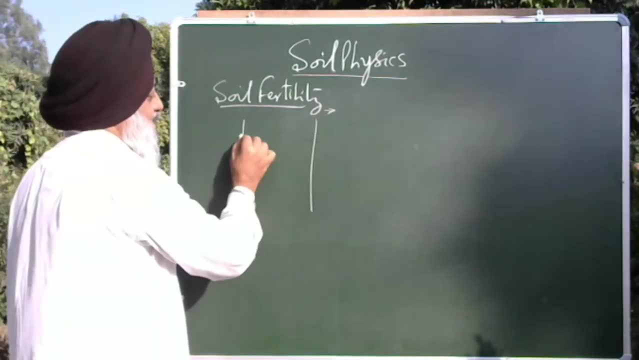 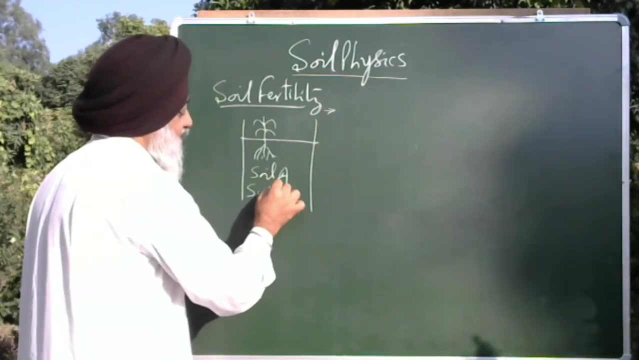 and then making it available to the plants. So I will simply explain the importance of soil physics by giving three examples. So first of all, say that soil, this is soil A, and here you have a crop plant growing and this soil has sufficient nutrients. 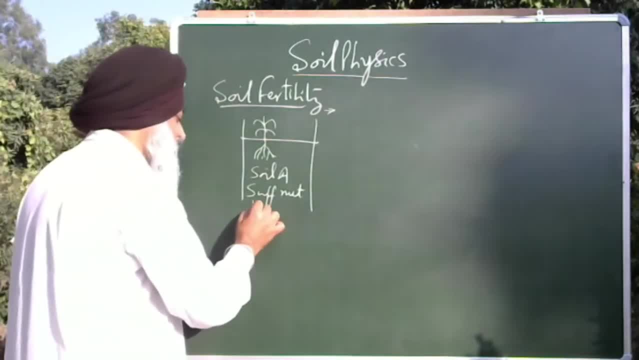 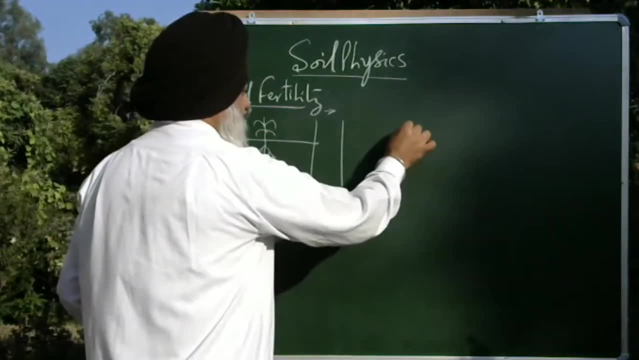 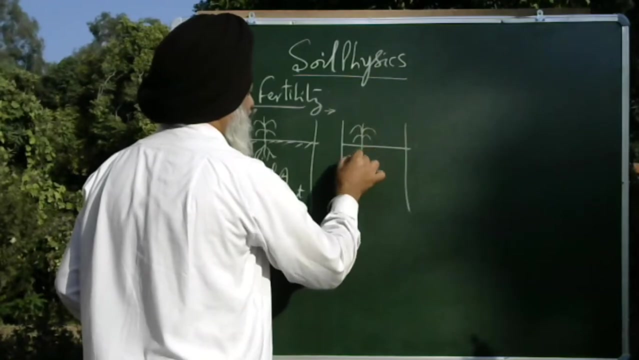 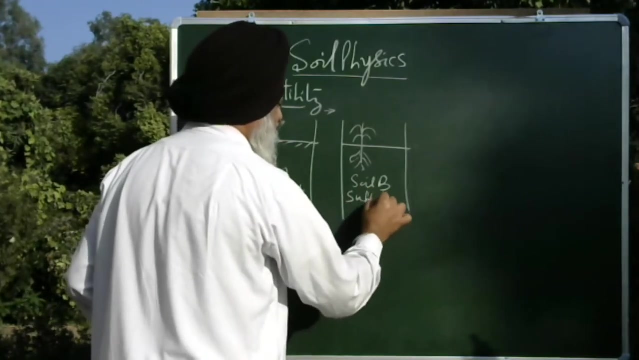 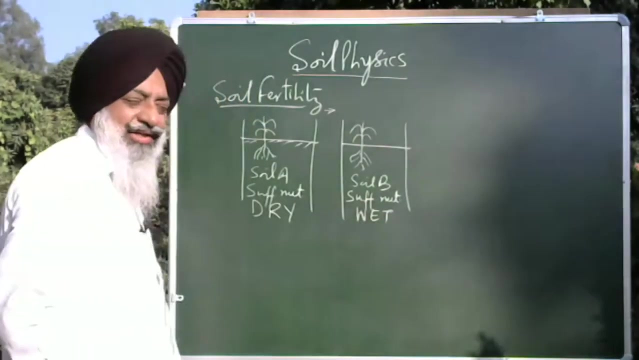 present in it, but at the same time it is a dry soil. Then we have another situation, that is, soil B, again with a crop plant with sufficient nutrients. but this soil is wet. When I say wet, it means it is more or less saturated soil: all the pores are filled with. 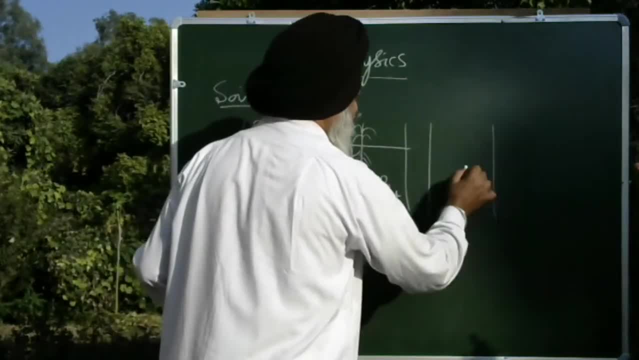 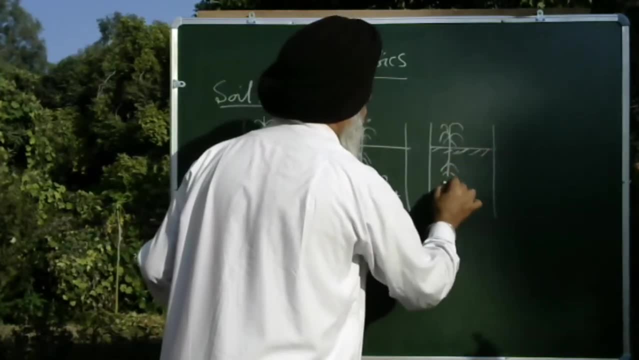 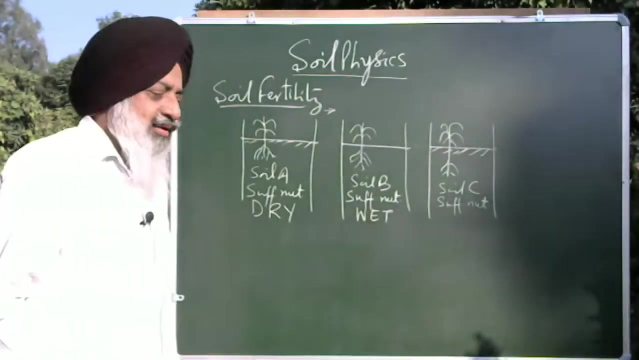 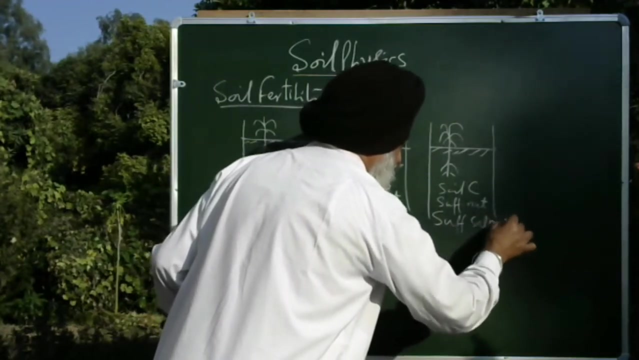 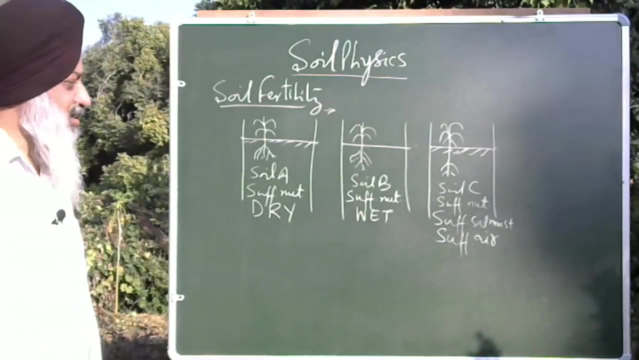 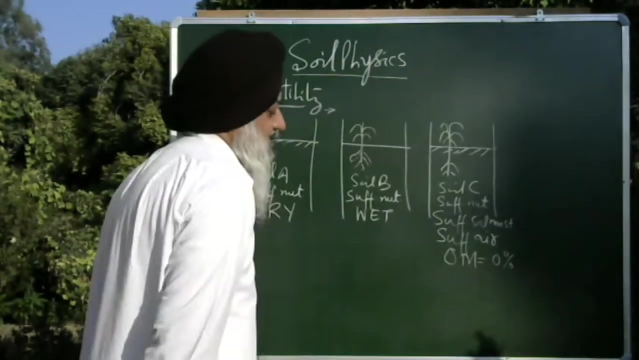 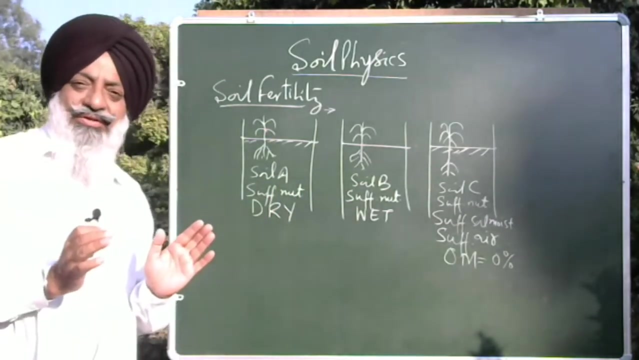 water. And then I will have a third situation. let us call it as soil C, which has sufficient nutrients, which has sufficient soil moisture, which has sufficient air in it, But it is organic matter content is 0 percent. Now see soil A. nutrients are present in sufficient quantity, but these nutrients are 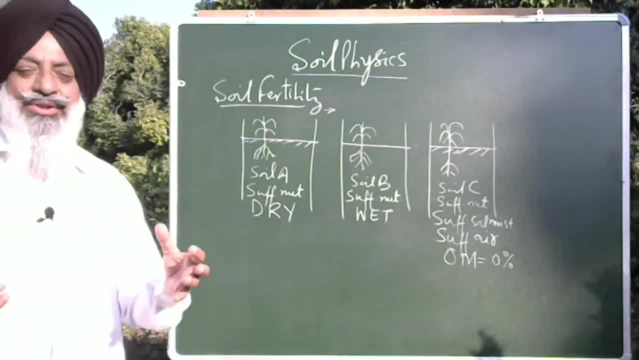 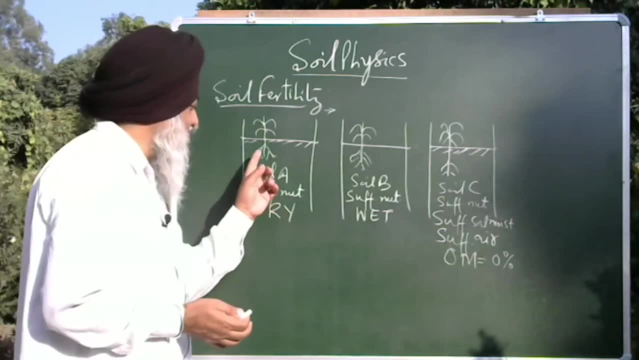 not available to the plants. The plant is not able to take up these nutrients from the soil, The reason being that the nutrients are always absorbed from the soil by the root. here in this soilosaat. Then we have h soci наверное Harryф er an đ Theresahand, nord Miputag, Chili, Darwin, Mas inevitable. its organic matter contentkin 10,0 %- now See South A. nutrients prendres on the soil, but these nutrients are not available to the plant. the plant is not able to take up these nutrients from the soil. the reason being: the nutrients are always absorbed from the soil by the root. here, see soil A. nutrients are always absorbed from the soil by the root. here it is an important element for the soil. 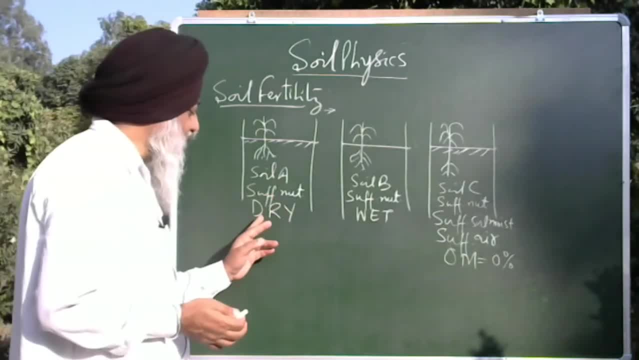 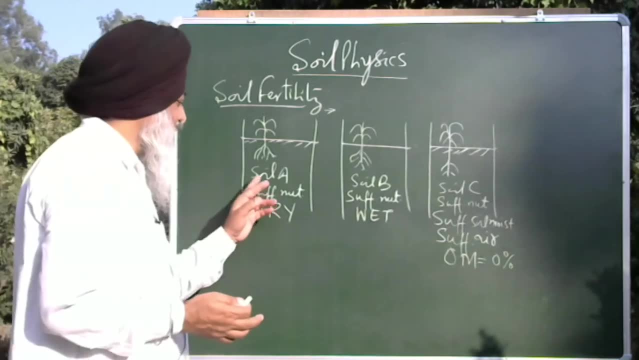 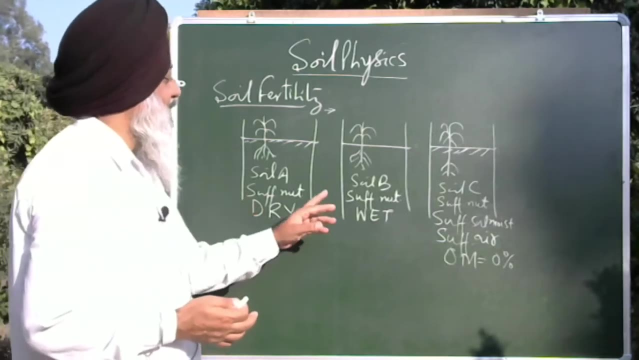 in the form of soil solution, but here we do not have any moisture. the soil is dry, So no matter how much nutrients are present in the soil, but these will not be taken up by the plant because there is not sufficient moisture in the soil. 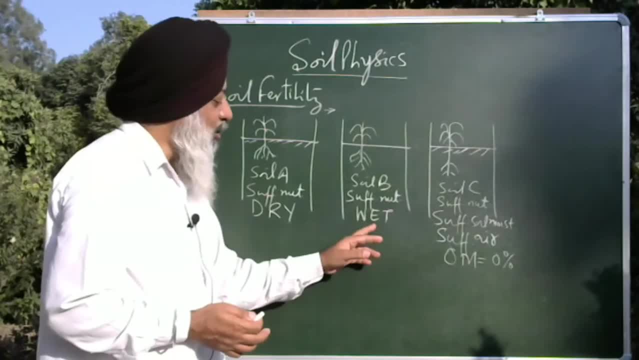 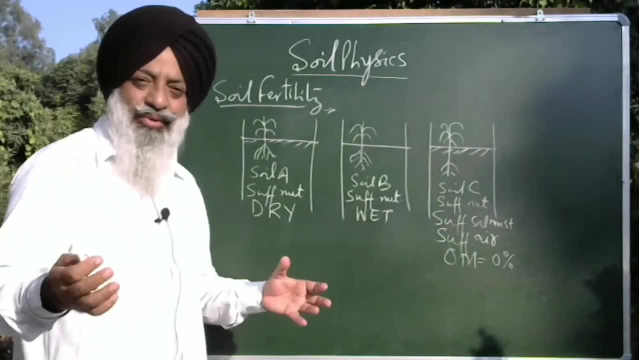 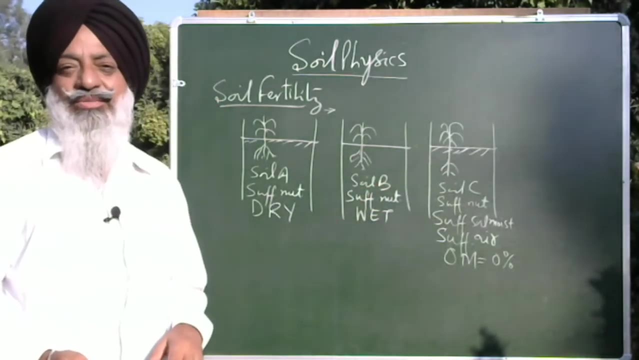 Coming to situation b: sufficient nutrients. moisture is, I should say, too much of moisture. moisture is too because I said, it is saturated soil or the pores are filled with water, so that means there is no air, and still the nutrients are not available to the plants. The plants, in fact, are not able to take up the nutrients from the soil, The reason being there is no air in the soil. so, in the absence of any air, the roots are not able to breathe properly. and if roots cannot breathe, they will not have oxygen. 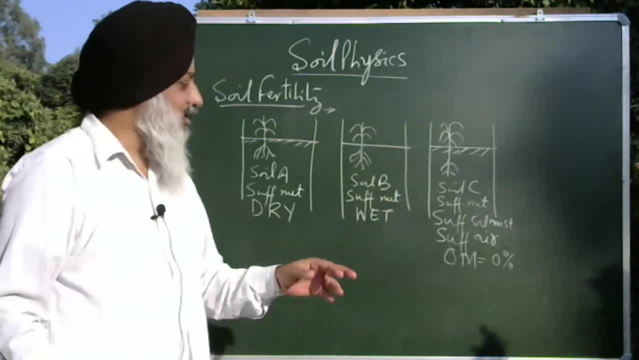 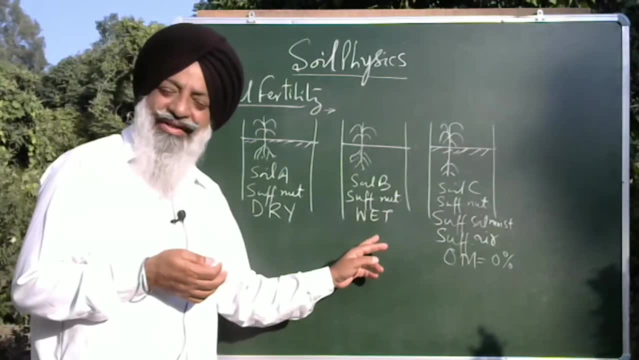 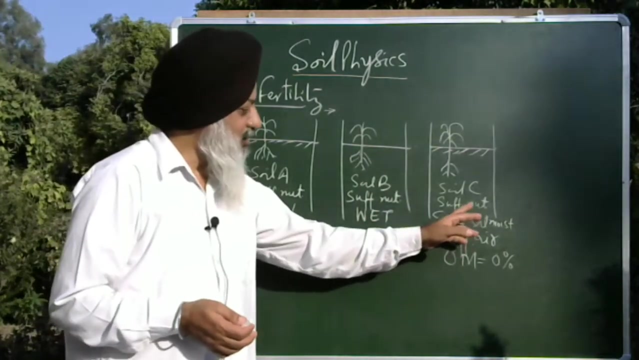 to take up nitrogen, phosphorus or potash from the soil. So that is the reason: Dry conditions: nutrients are not available. too wet conditions: nutrients are not available, and here the nutrients may be available because sufficient nutrients are there, sufficient. 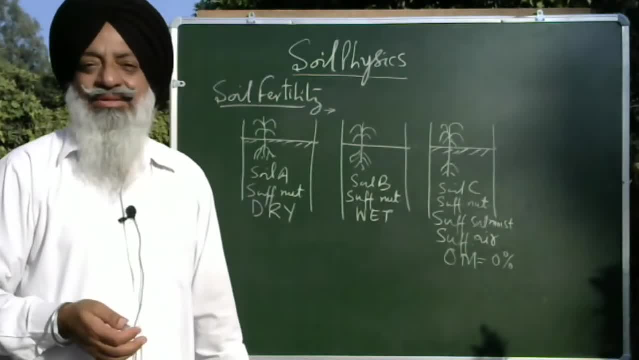 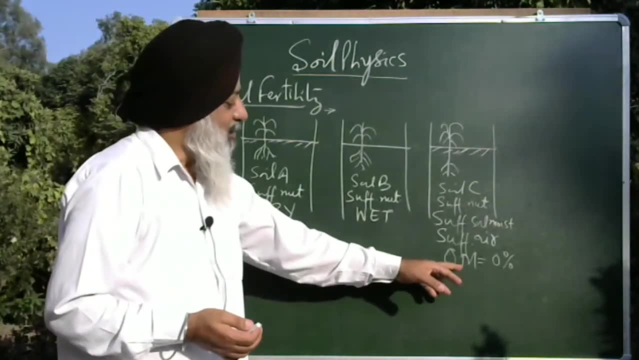 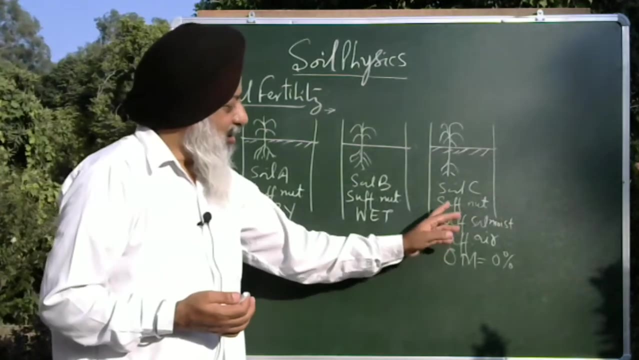 moisture is there, sufficient air is there, but because of the presence, absence of organic matter, these nutrients are, I should say, may not be fully available to the plants. because of the presence of organic matter, these nutrients are, I should say, may not be fully available. 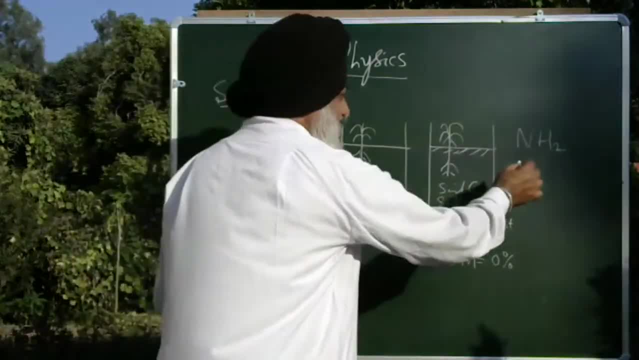 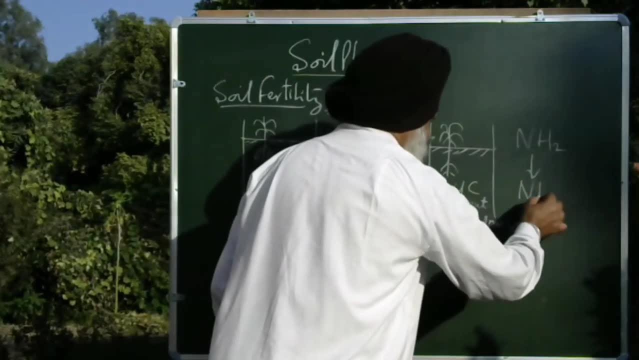 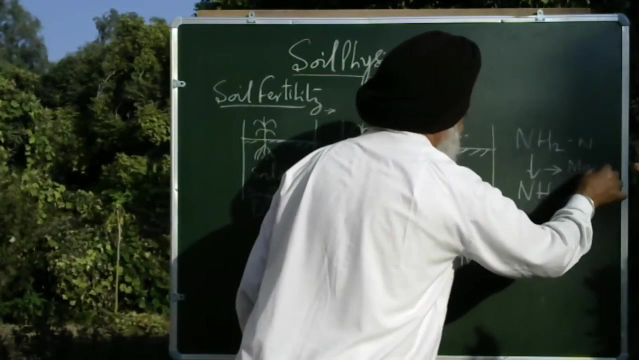 So you are adding the nutrients in the form of amide NH2, say nitrogen. we add urea. urea is amide group and this amide is not taken up directly by the plant roots. this is first converted into ammonical nitrogen and this conversion takes place by microbes. you can call it. These are, in fact, broadly these are called as ammonifying bacteria. and if your soil is saturated, some plants- like in agriculture we have the rice plants- which have the capability to take the nitrogen in ammonical form, because ammonical form will always be present under 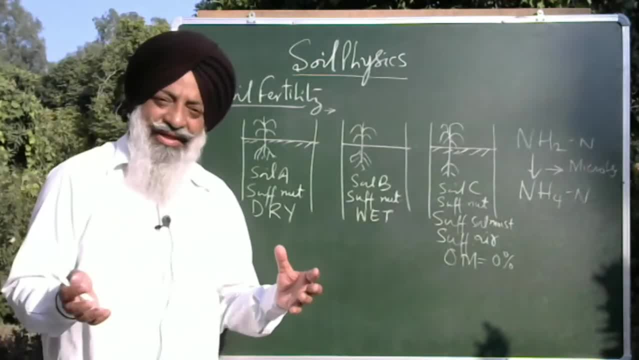 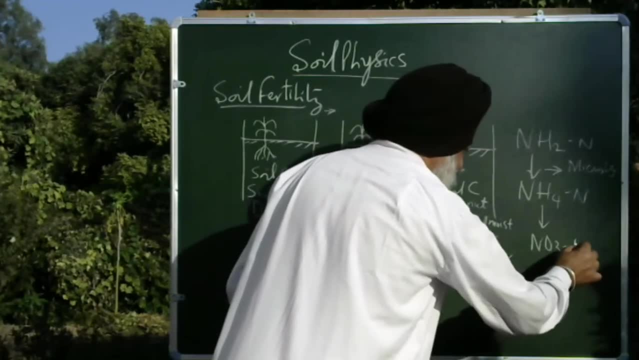 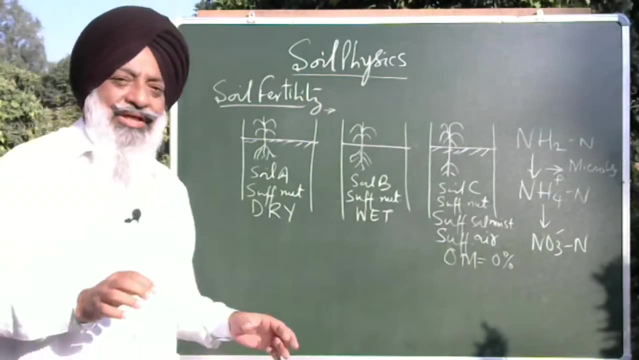 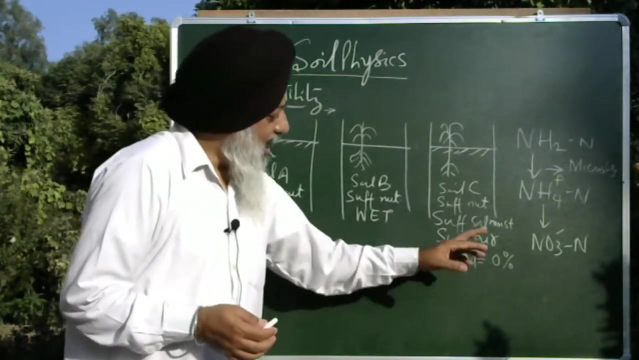 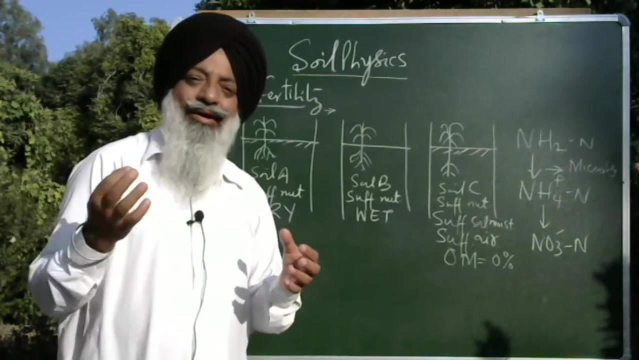 reduced conditions and in submerged rice fields reduced conditions are there, but other than rice crop plants take nitrogen in the form of nitrate and this nitrate nitrogen is converted by nitrifying bacteria. So, as I said, bacteria or microbial population will be there in the soil only if they have foods to grow and their food is. 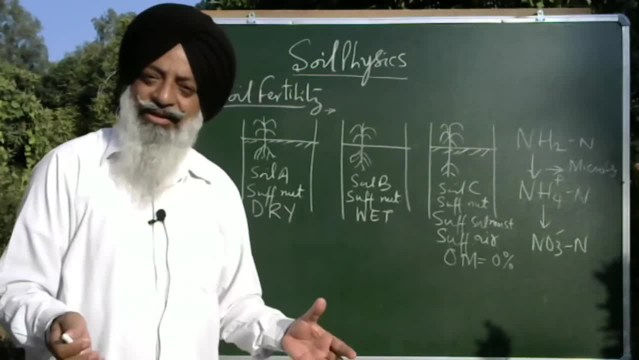 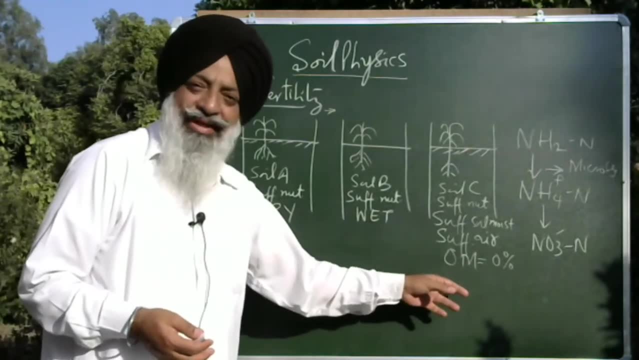 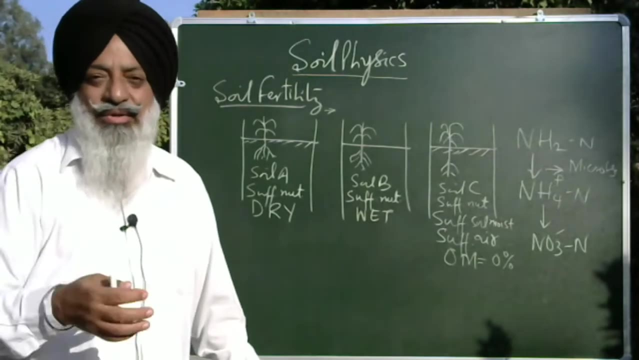 organic matter. So if you do not have organic matter into the soil- say we are assuming that it is 0%- then this means there will not be any food for the microbes and microbial population will be low. So, though nitrogen is present in the soil, you are adding urea into the soil. still that urea may not be available. 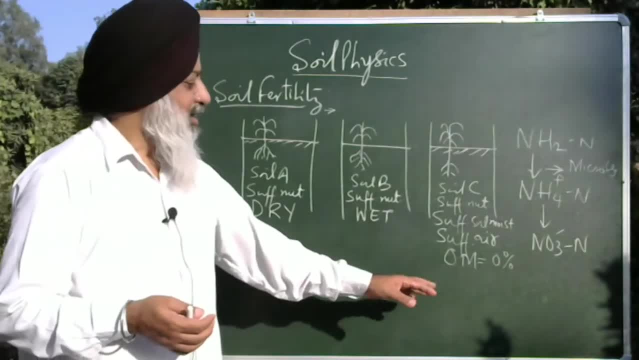 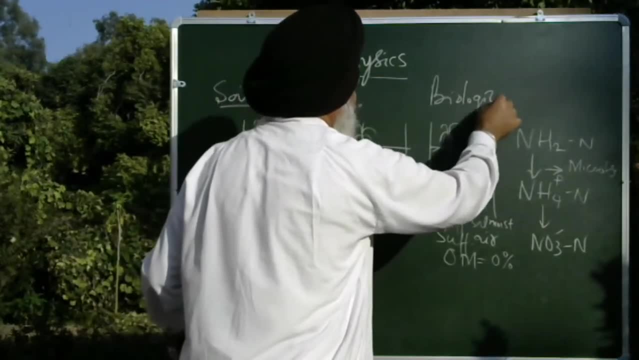 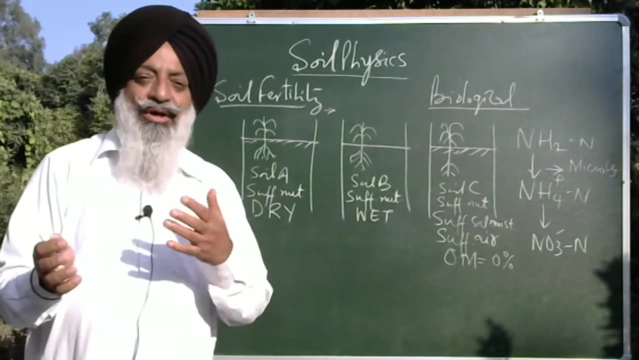 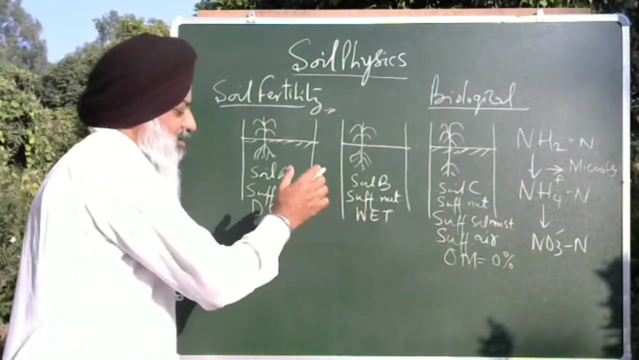 that nitrogen may not be available to the plants in the absence of So. here it shows that this is the biological fertility of the soil. So for a soil to be fertile we should have sufficient population of microbes and here optimum conditions of moisture, optimum conditions of air in the soil. it is, it is determined by the soil physical. 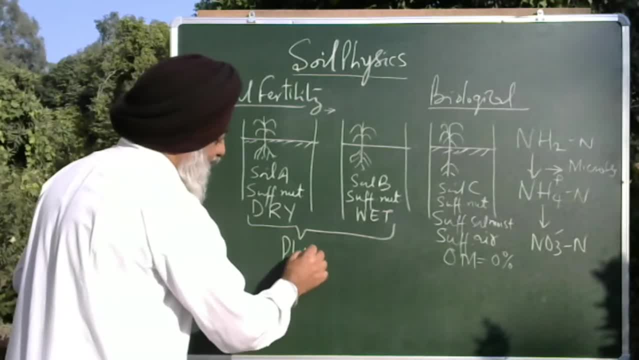 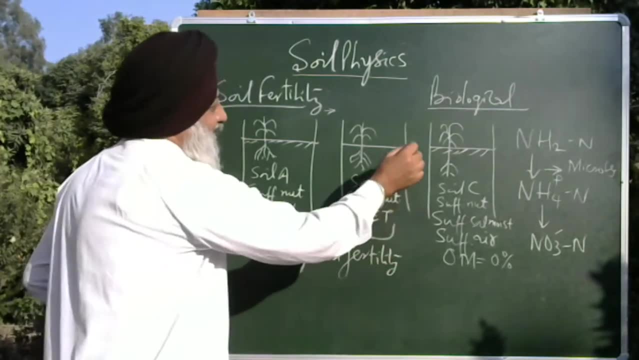 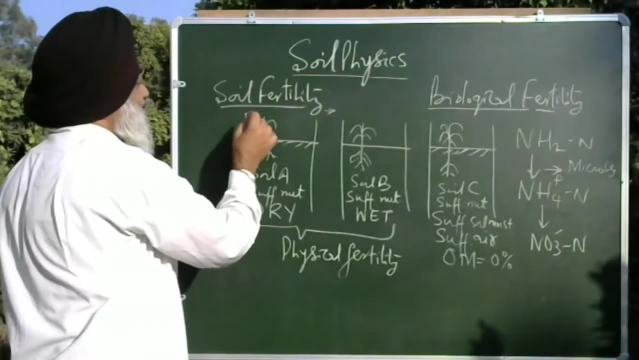 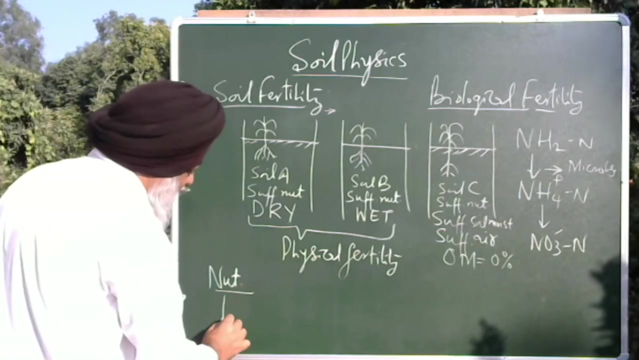 environment. So we call it as physical environment, or you can call it as fertility of the soil, and here it is biological fertility of the soil and the presence of nutrients itself. you call it as chemical fertility of the soils, Not only nutrients, but pH, etc. even cation exchange capacity. so this determines the 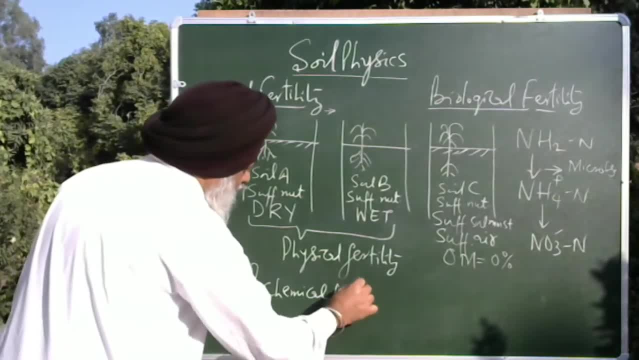 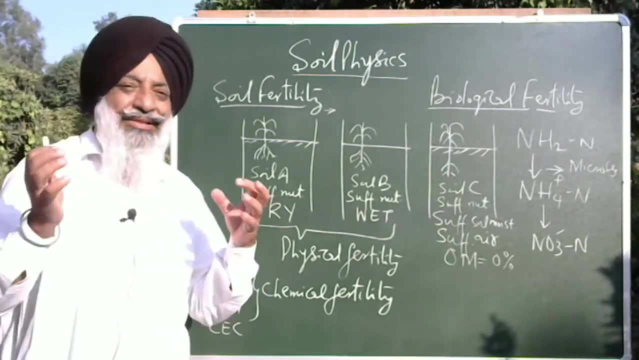 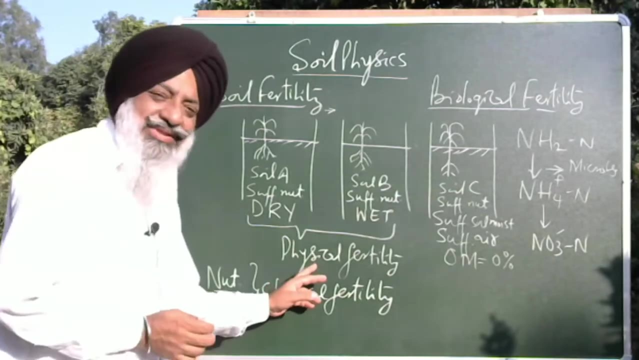 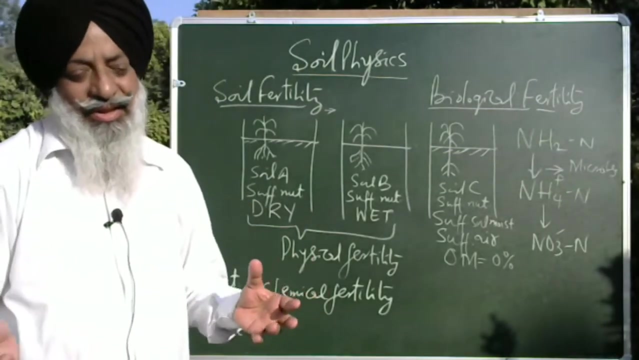 chemical fertility. What I mean to say over here is that soil fertility- as soil is said to be fully fertile if it has very good chemical fertility, if it has very good physical fertility, a very good physical environment and there is microbial population, good biological fertility. So in fact, when we say soil fertility it has three components: chemical- 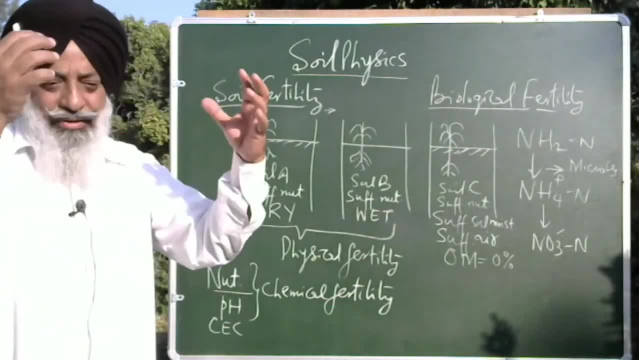 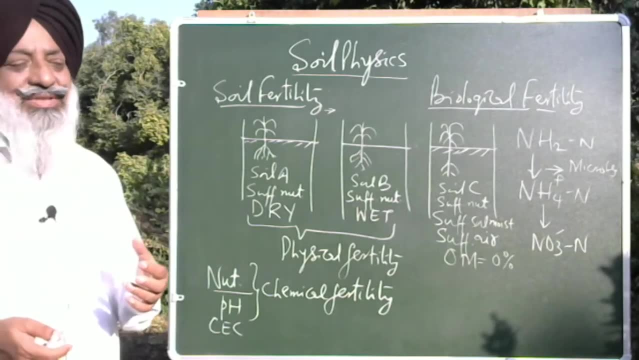 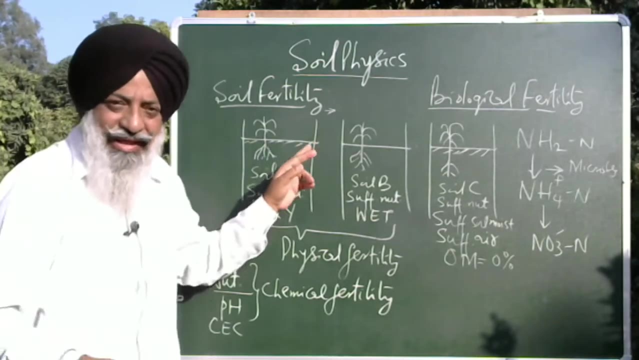 fertility, physical fertility and biological fertility. So all these together determine the fertility of the soil. and now, if I have to redefine the fertility of soil, I will say it is the ability of the soil to sustain plant growth, to sustain crop growth, and that is. 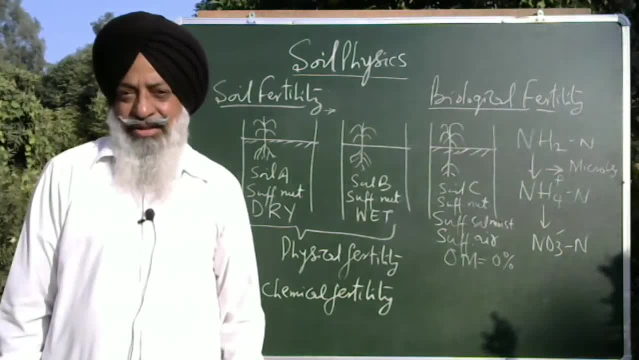 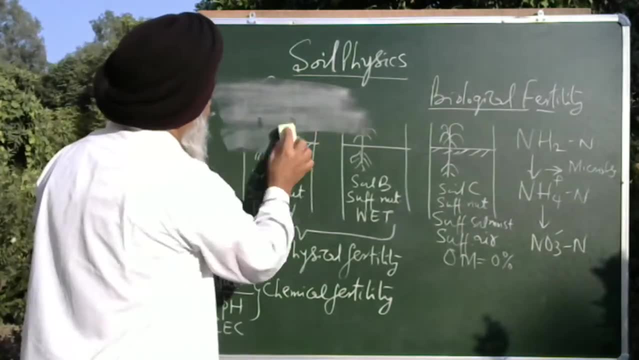 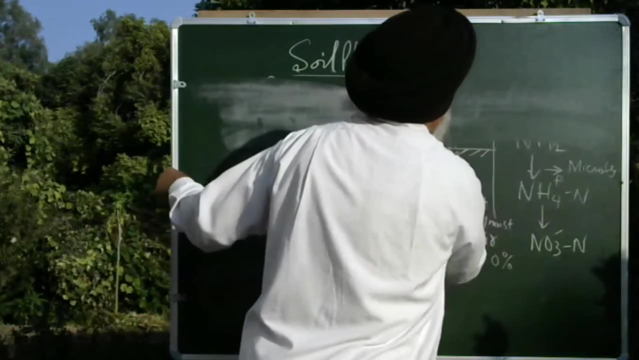 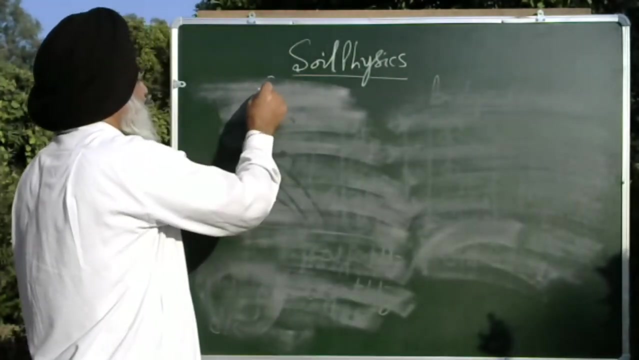 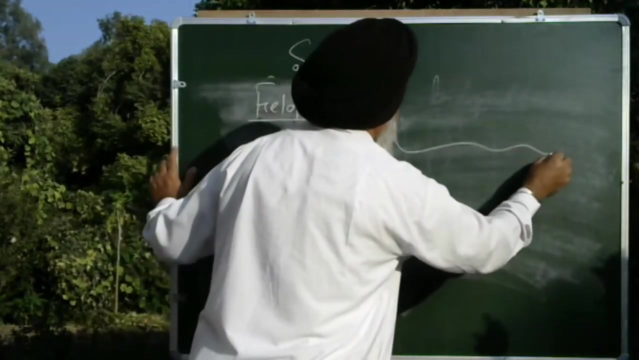 why soil physics becomes important. Now I will give you another practical example where soil physics is very, very important, and that practical example is prevalent in, most of you know, the intensively cultivated fields. Let me give you an example that you have a field, say, here. it is the field and you have 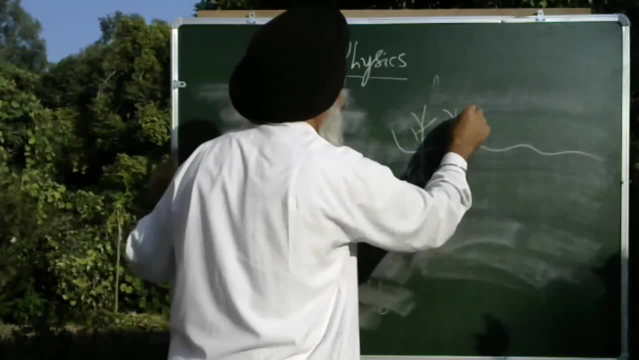 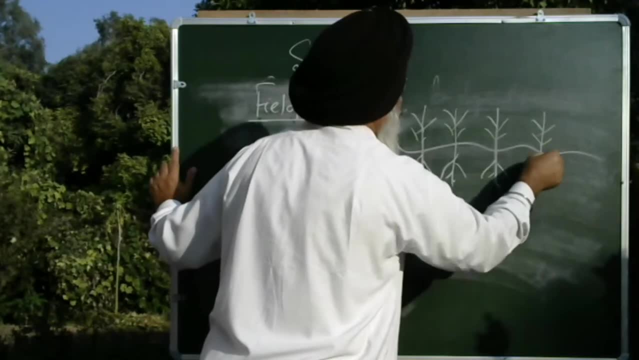 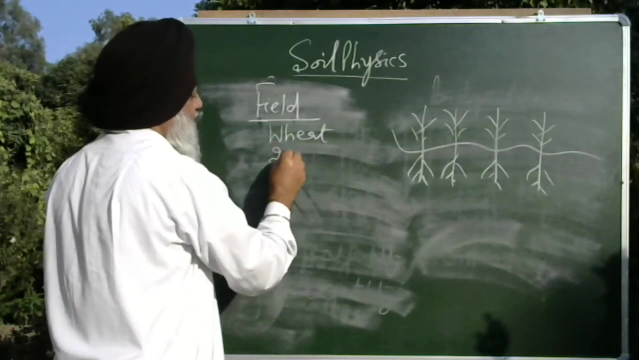 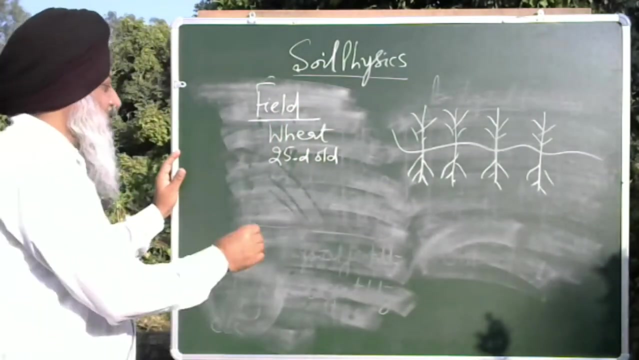 the crop plant, and this crop plant is, in fact, the wheat growing over here. So basically, this is the wheat growing over here. So basically, this is the wheat growing over here. So basically, it is a wheat field. So crop is wheat, its age is 28 or you can say 25 day old. 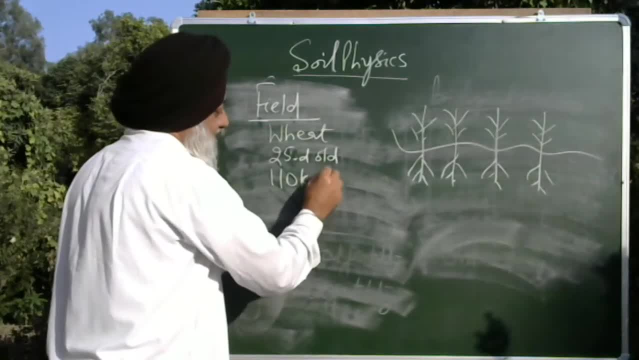 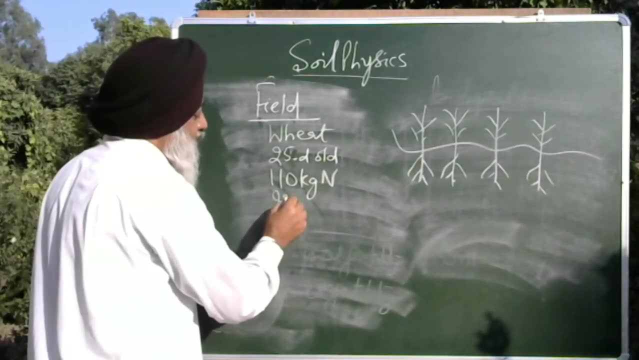 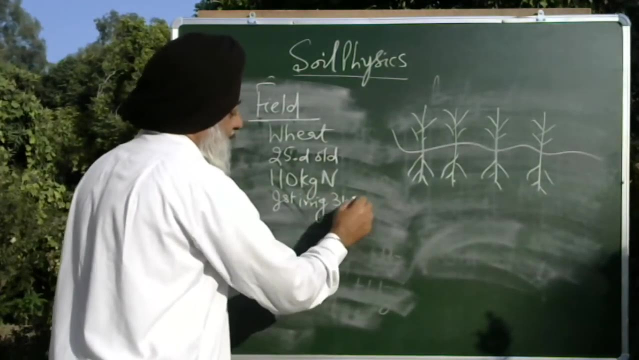 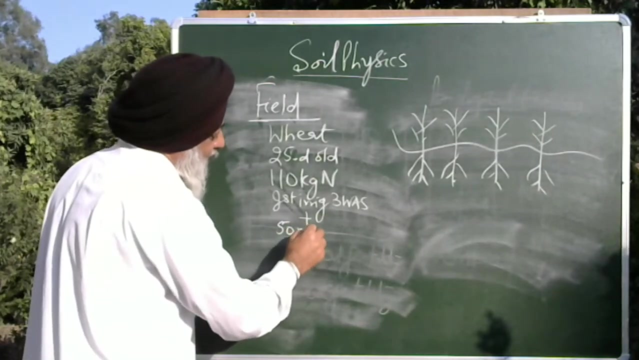 We have applied 110 kg of nitrogen to this field and then we have also given first irrigate and then we have also given first irrigation to this crop. after three weeks, after sowing And after first irrigation, what happens? that 50 mm of rainfall occurs within two to three. 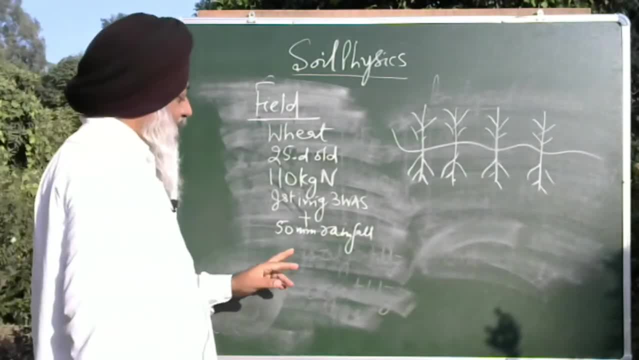 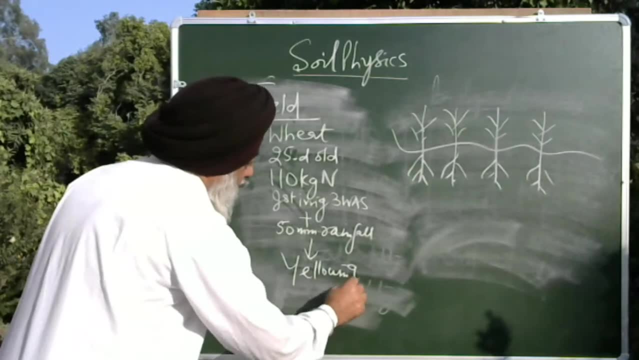 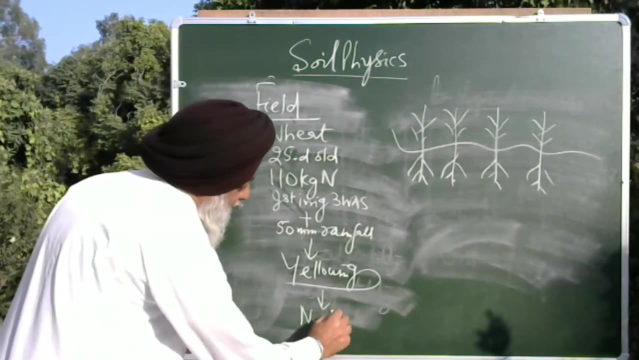 days of the irrigation. Now, after this, what happens that wheat plants? they show yellowing of the leaves. Now, after this, what happens? that wheat plants, they show yellowing of the leaves. And if we diagnose this yellowing, it is nitrogen deficiency. typical symptoms of nitrogen: 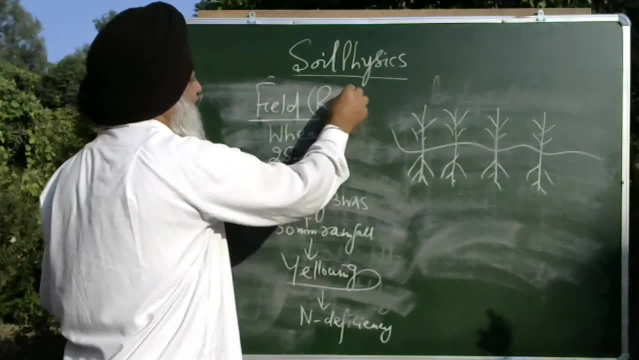 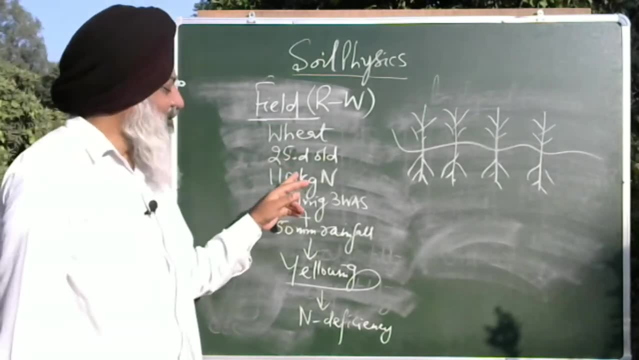 deficiency, And if we diagnose this yellowing, it is nitrogen deficiency. typical symptoms of nitrogen deficiency- And this field, in fact, is rice wheat field. That means the cropping rotation is rice and wheat. Now the question is: we have added sufficient amount of nitrogen in the soil? 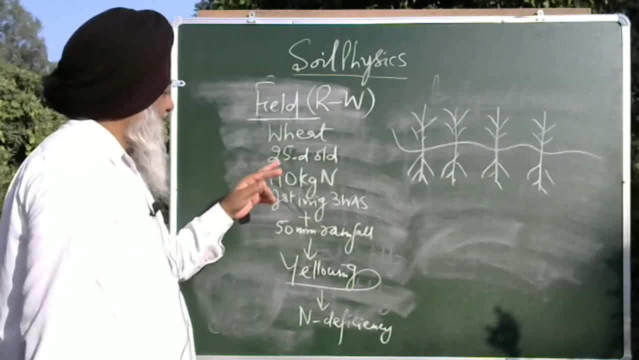 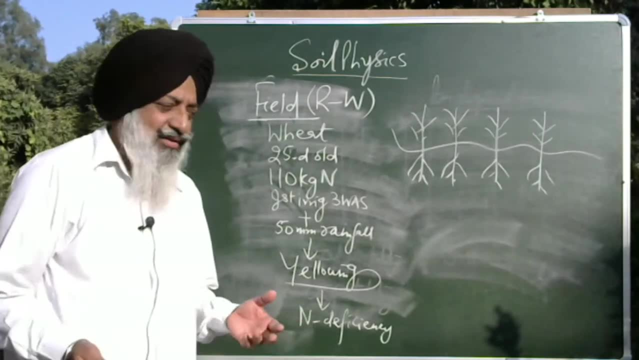 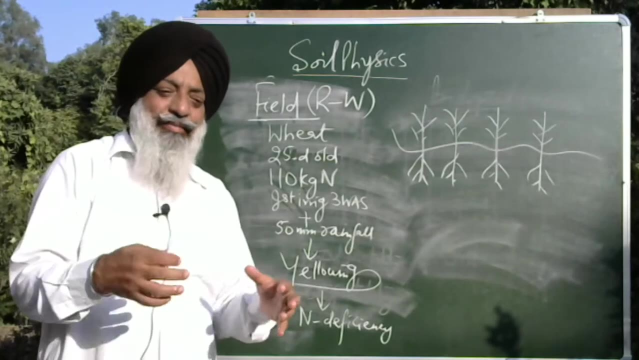 We have good amount of irrigation Crop. is there very good crop The plants? they are showing deficiency of nitrogen Why? The reason being it is a rice wheat field and you know, in rice crop we puddle the soil and puddling means it is wet cultivation. 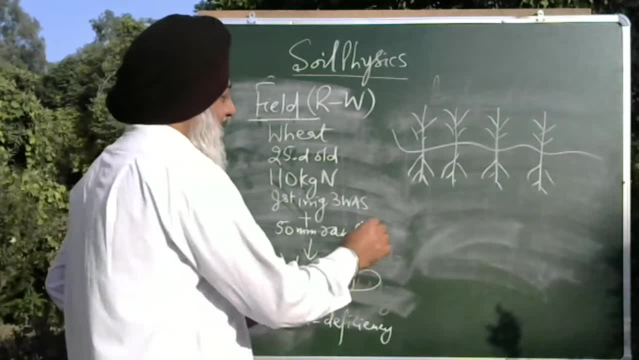 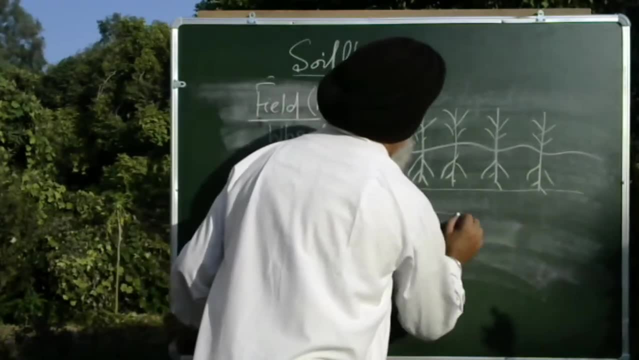 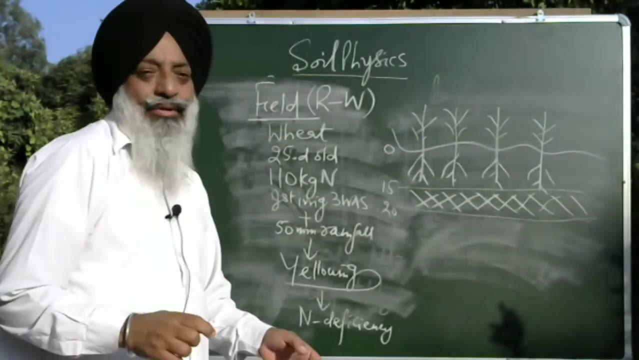 So when you are puddling the soil, the wetness is there at some depth. If this is 0 centimeter, at 15 to 20 centimeter depth a sort of compact layer is formed because you know When this proctor moisture content is there. proctor moisture content, in fact, is the moisture. 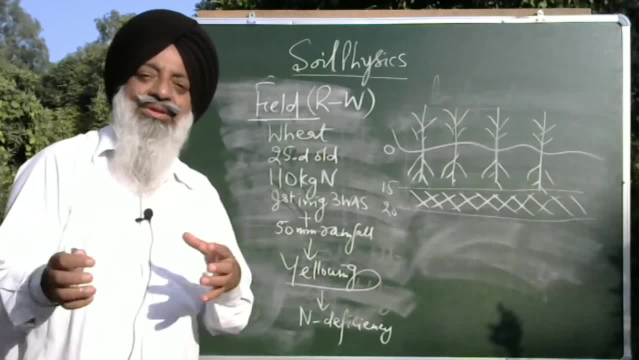 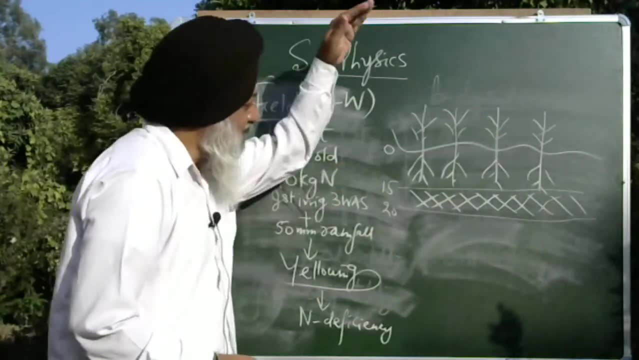 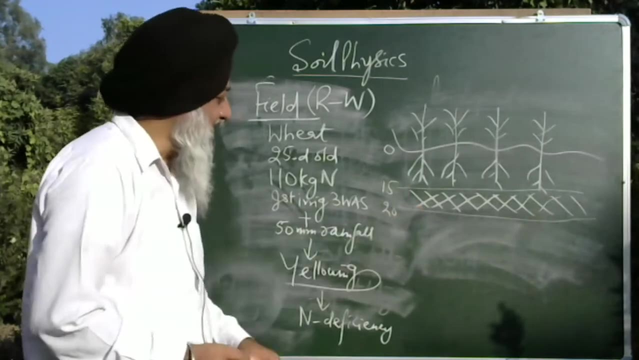 content of the soil at which the compaction can be done to the maximum extent. So, because the soil 0 to 15 centimeter is wet, you are puddling it. So with the pressure of the tires, this compaction takes place at 15 to 20 centimeter depth, and 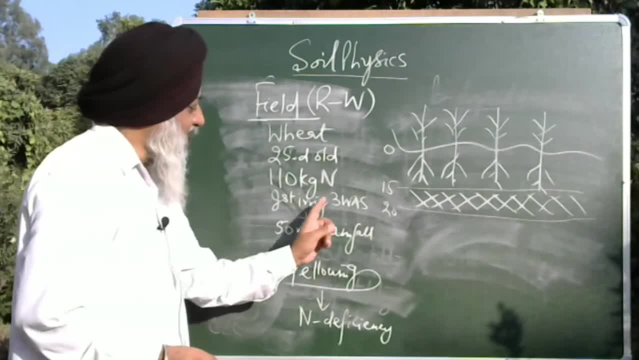 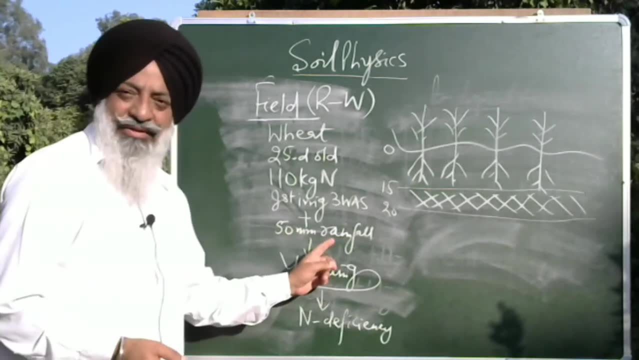 a hard layer is formed. Now what happened? The farmer applied first irrigation. Now what happened? The farmer applied first irrigation at 21 days after sowing. Then, after 2 to 3 days, there was 50 millimeter of rainfall. 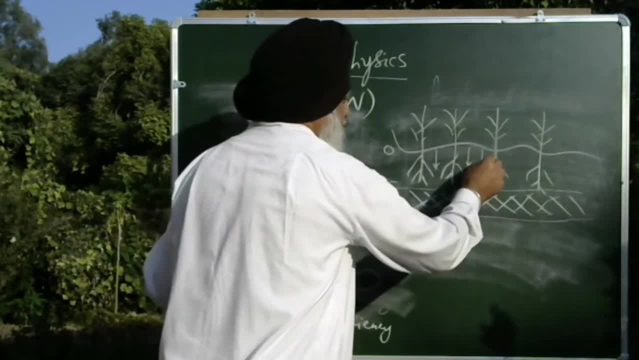 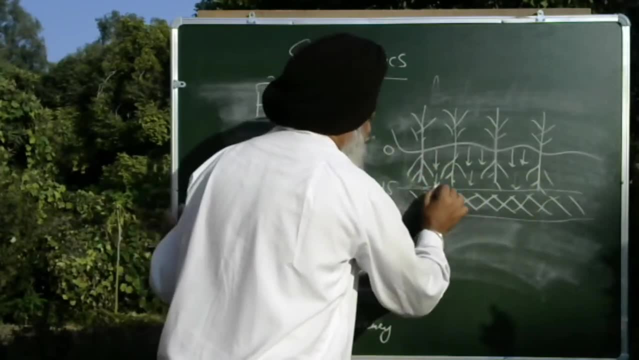 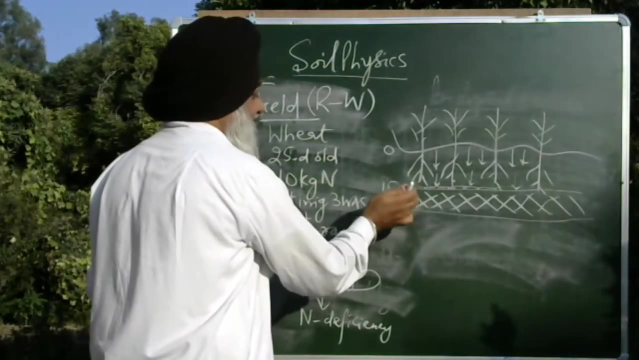 So what happened This water, when it entered into the soil and it reached at the boundary of the hard layer? this water, its movement, stopped over here for some time. At the boundary of hard layer, this had 15 to 20 centimeter and the low ball density. 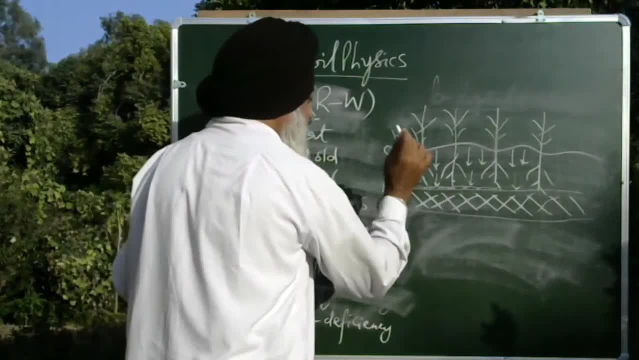 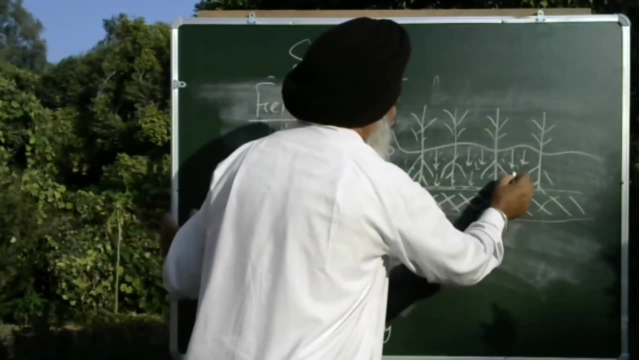 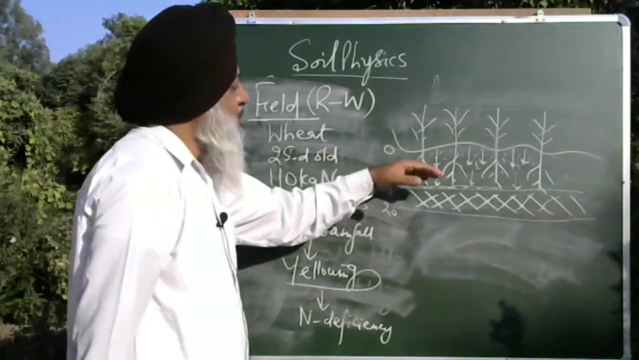 layer above. So with the result: for some time there is temporary water logging conditions, or you can say temporary saturation of 0 to 15 centimeter, And since the crop is 25 days old, so most of the roots are concentrated only in 0 to 15 centimeter layer. So when all these pores get filled- 0 to 15 centimeter zone gets saturated, Then the roots are concentrated. So when all these pores get filled- 0 to 15 centimeter zone gets saturated, Then there is absence of oxygen. 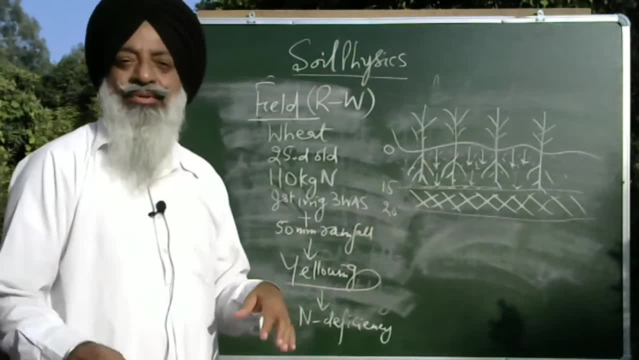 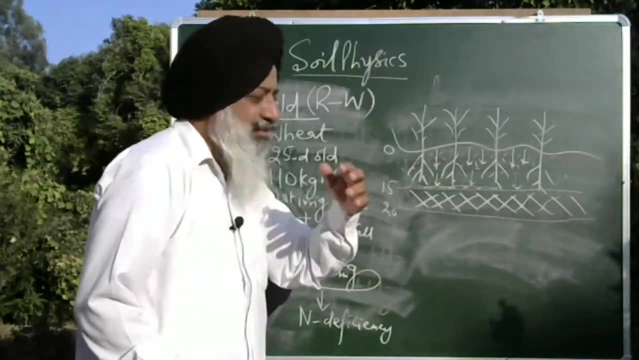 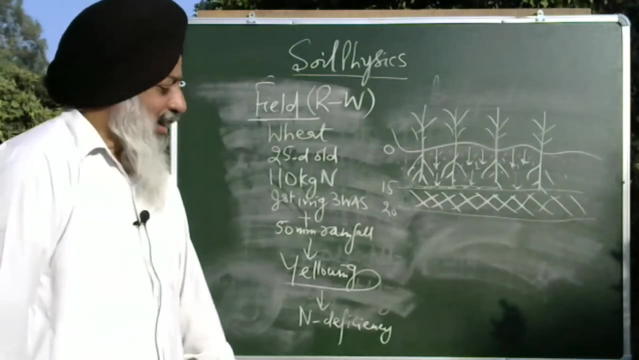 And when oxygen is not there, the roots are not able to take up nitrogen from the soil. because roots cannot breathe, Roots do not have the energy to take up nitrogen from the soil. With the result, the plants. they show typical nitrogen deficiency symptoms. 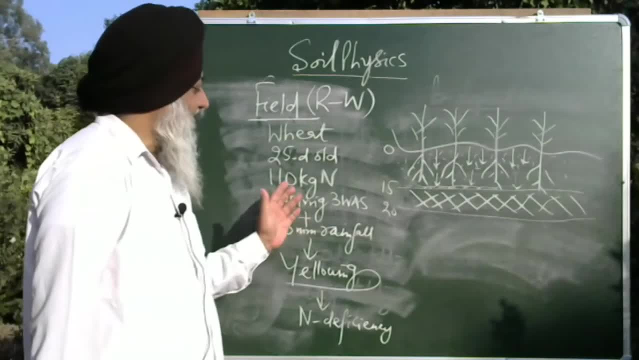 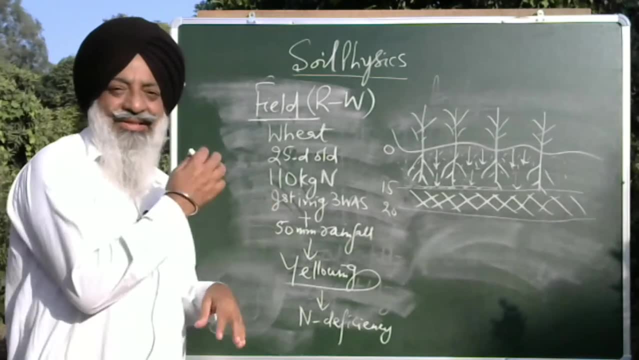 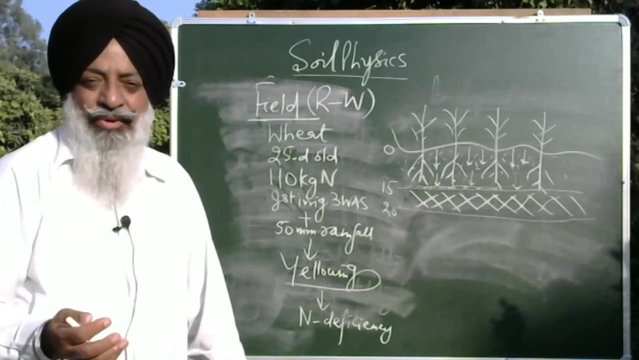 And at Punjab Agriculture University we have diagnosed these many times. So if this situation happens, that after first irrigation There is immediately rainfall, then the farmers they come to plant cleaning of PAU and they are not able to diagnose that why it happened. 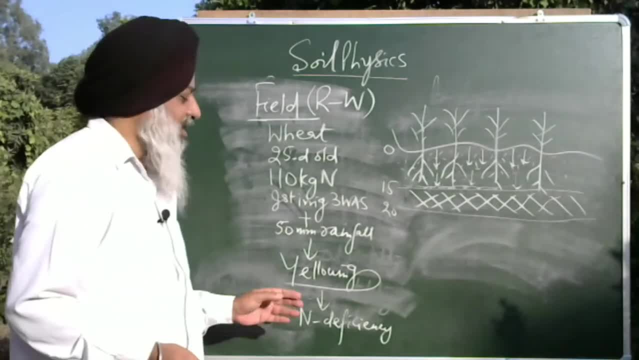 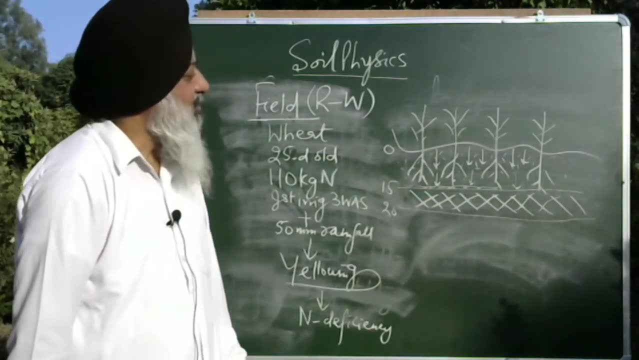 Farmer says that he has added sufficient nitrogen in the soil. Still nitrogen deficiency is there. So it is because of this reason, And once we diagnose it, then we recommend to the farmer to spray the solution of 2 to 3 percent solution of urea. 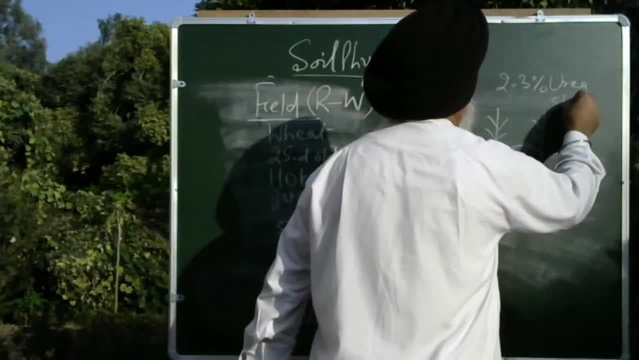 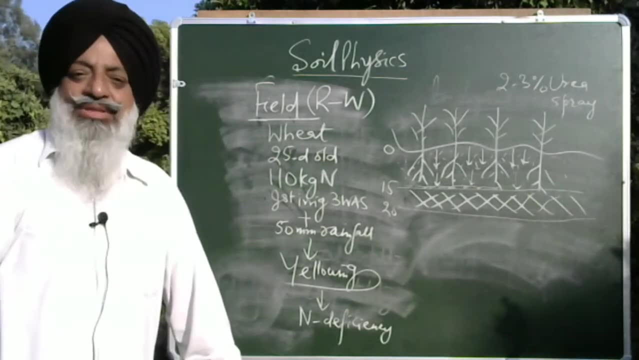 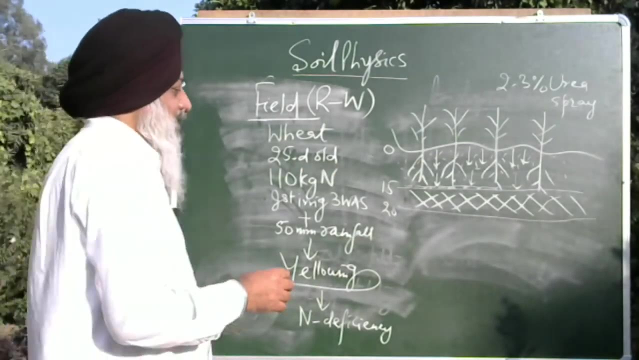 So that is the reason. So that is the reason, So that the plant leaves are able to take up nitrogen directly from the leaves. So this is a practical example which the farmers they face, And many a times it has been observed that at one time the losses reduction in yield. 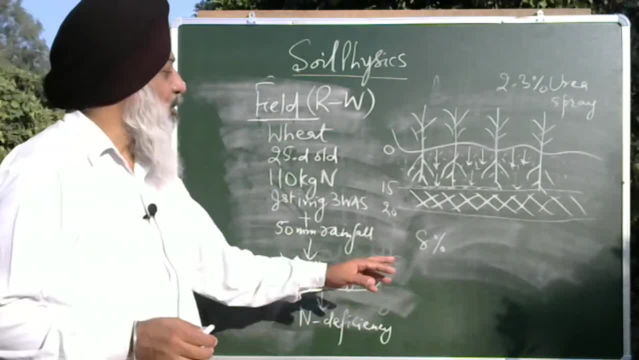 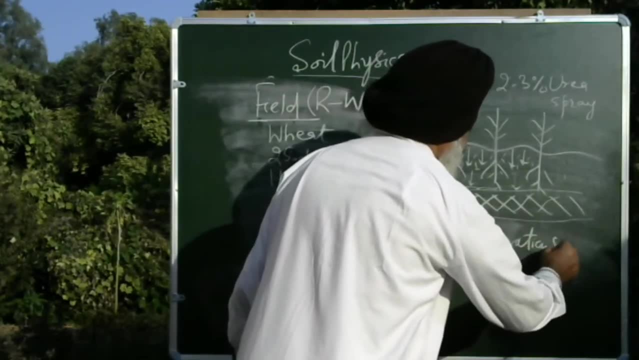 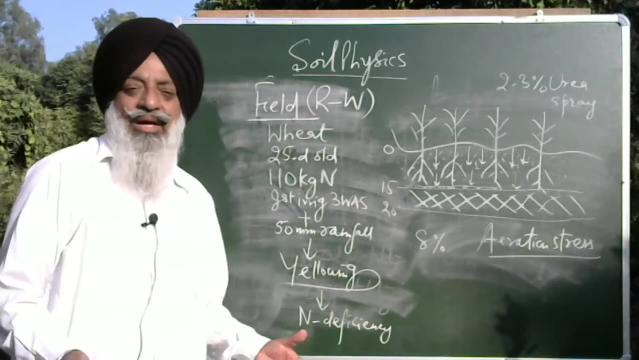 has been to the extent of 8 percent. because of this problem, We call this as aeration stress, So that means the plants are feeling the stress of aeration. The plant roots have not sufficient, you know, air present in the soil and because of this, 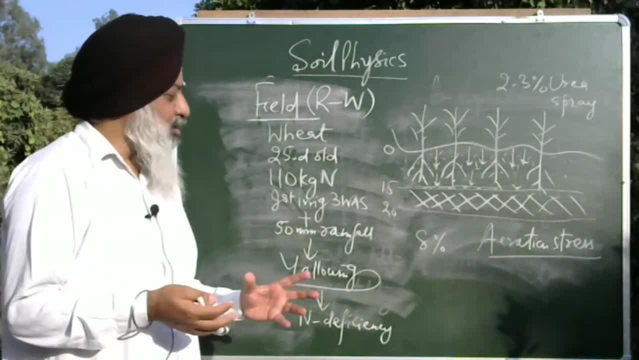 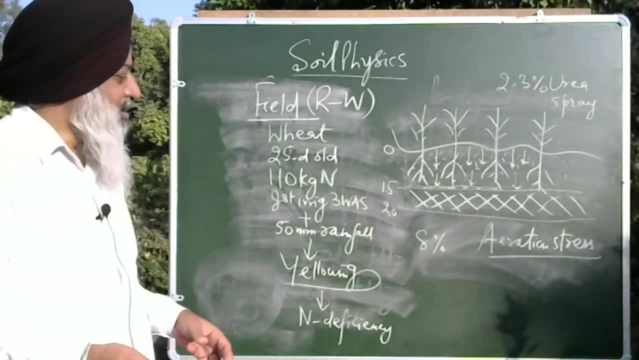 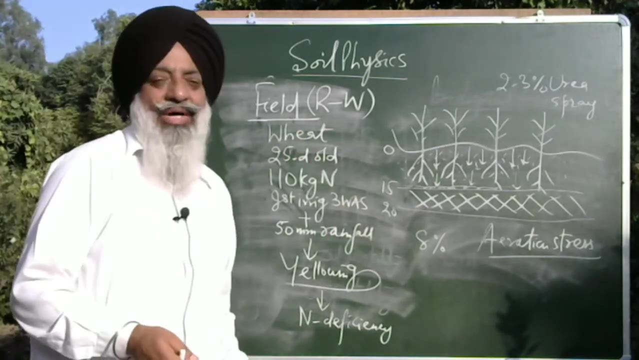 So if this example is clear to you, this typically shows the role of soil physics, that how important soil physical environment is. Otherwise, whatever you do, whatever amount of Nutrients you add, if soil physical environment is not good, it will hamper the crop yield. 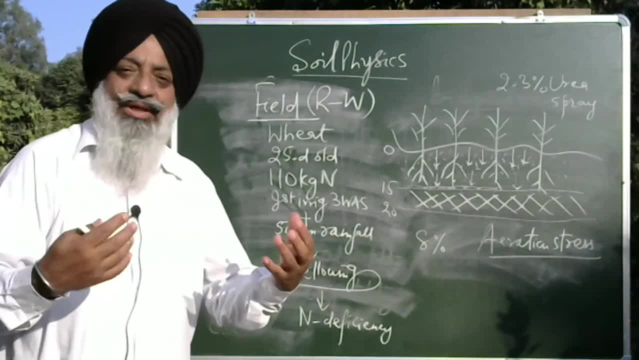 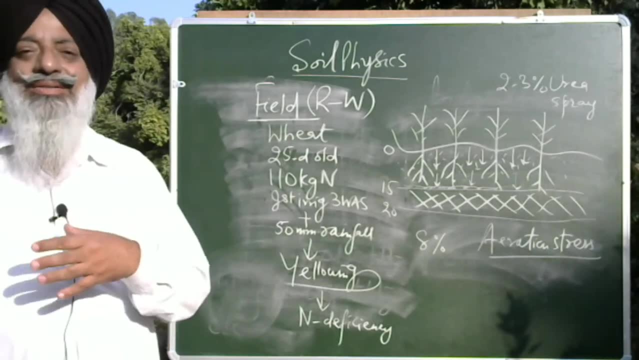 So I hope that the things are clear now and you can yourself now write that. why soil physics? what is the importance of soil physics? why it is important in agriculture. Thank you very much.